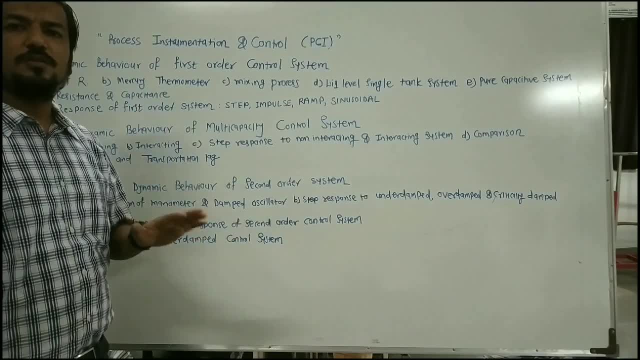 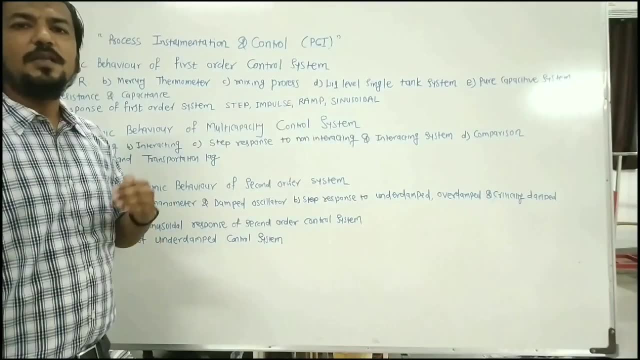 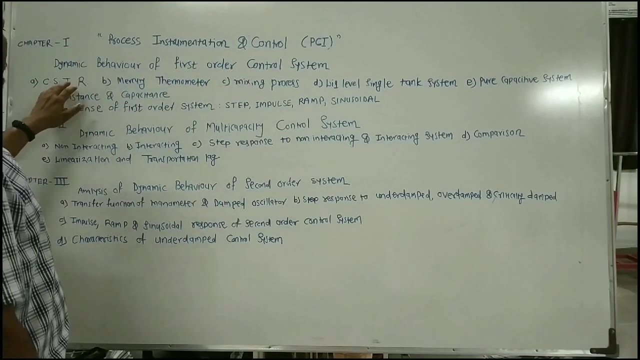 What you have to do? You have to determine the transfer function of the first order system and then you have to provide some input to the first order system to study how the first order system reacted with respect to time. That is the response of the first order system. So here the dynamic behavior of the first order control system includes following: determination of the transfer function of the following types of the system: 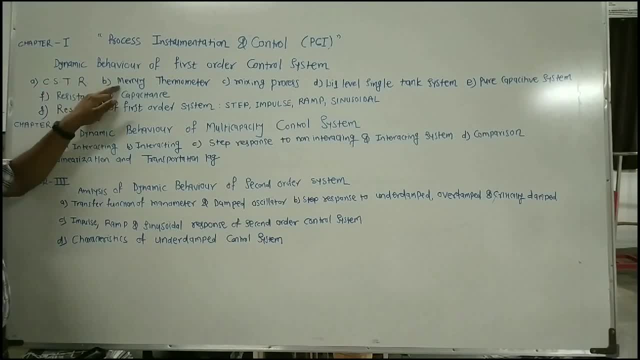 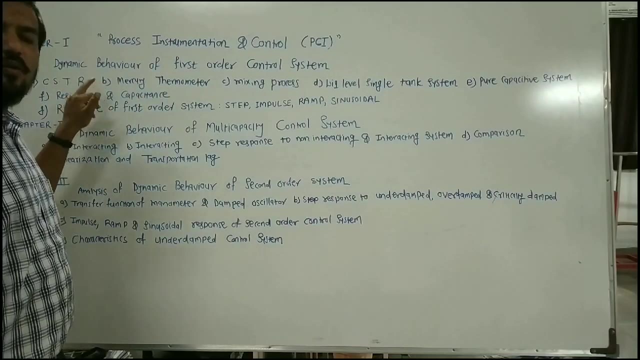 Very first is the continuous turn-tang heater. Mercury thermometer Mixing process, Liquid level, single-tank system, Pure capacitive elements. All of these 1,, 2,, 3,, 4,, 5,, 6 to 7 systems. you have to determine and you have to prove that these systems are the first order control system. 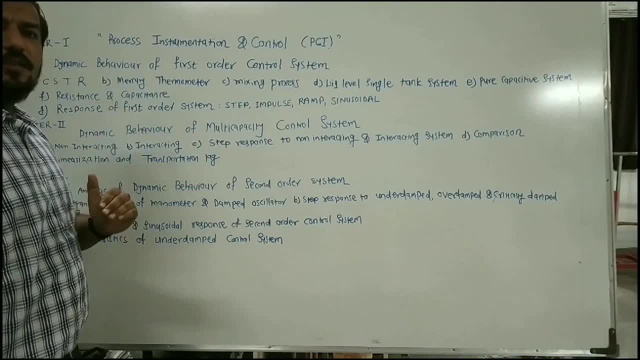 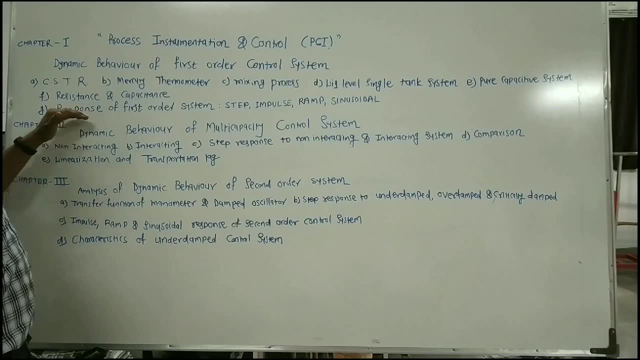 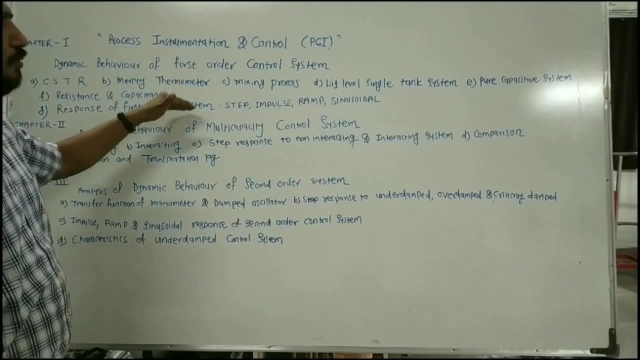 Once you have completed this, later on by considering this system, you have to provide the input to this system. They are called as the forcing function. So the latter part of this unit included response. Response of the first order system means this first order system, how they will be respond when you will give it an input like state impulse, ram and sinusoidal forcing function. 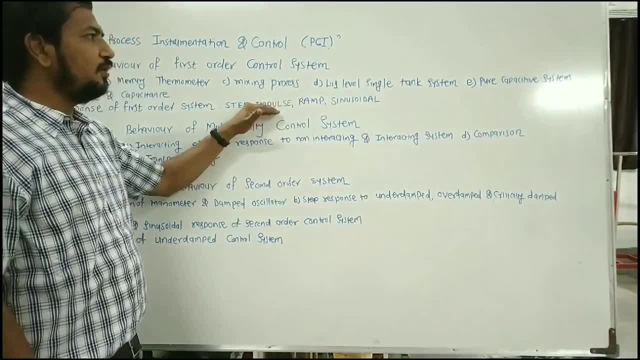 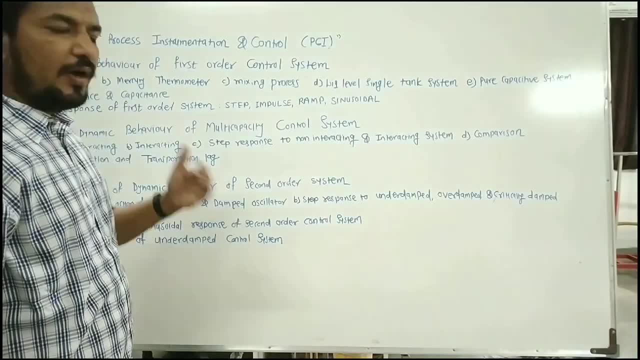 All of these are the four types of the forcing function which has been included, and you have to give to this first order system and study the response equation. Now, this is okay about the unit number 1.. What happens in the unit number 2?? 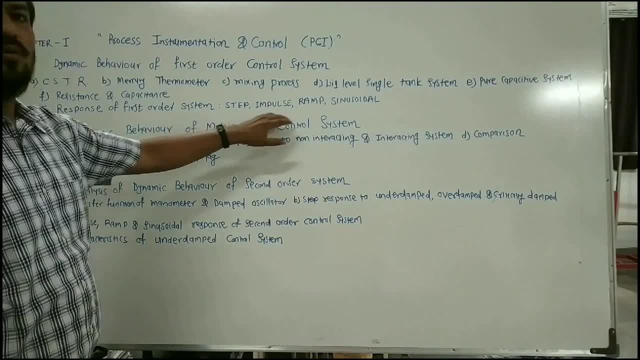 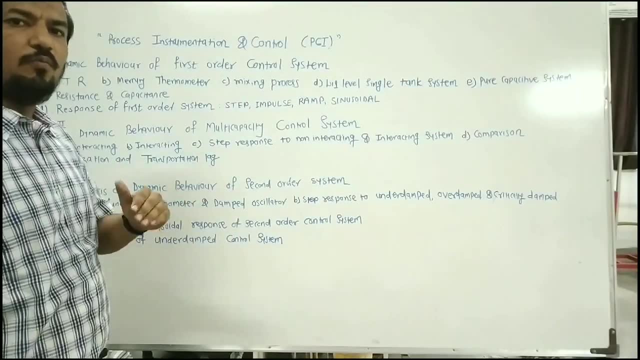 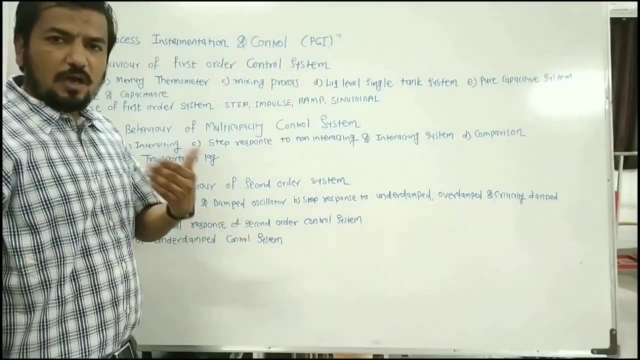 You have to study the dynamic behavior of the multi-capacity control system. So very first question is: what is the multi-capacity control system? Now, multi-capacity system is nothing but when more than one first order systems are arranged in a series. then how the system changes, its response and how the transfer function changes, that you have to study. 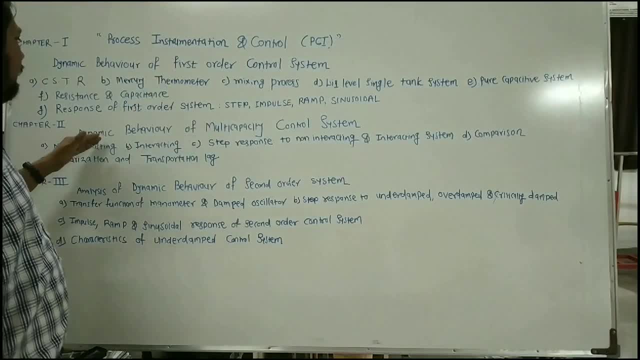 So already you have studied the first order system, So multi-capacity control system, this unit included. there are two types of the multi-capacity system which you can be arranged. Very first is the non-interacting. So in this unit you have to first provide the transfer function of non-interacting system. 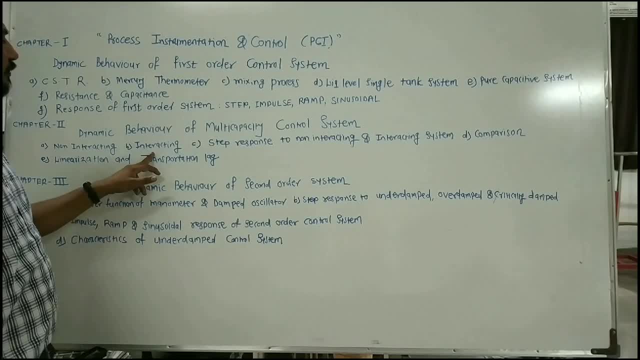 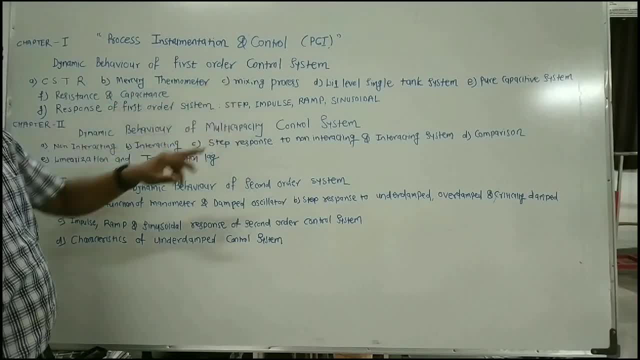 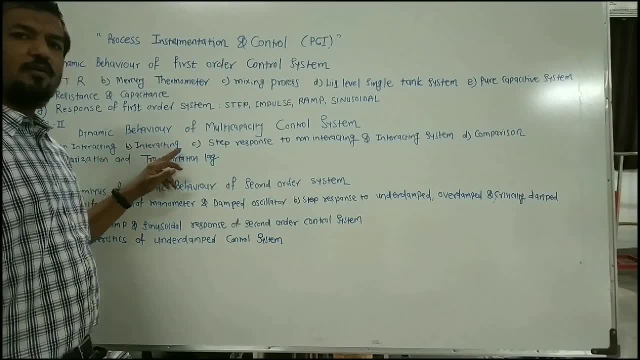 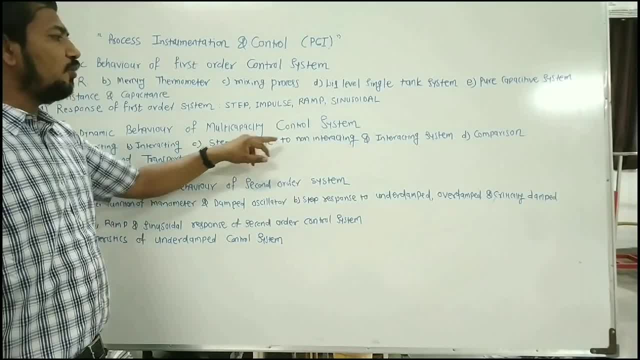 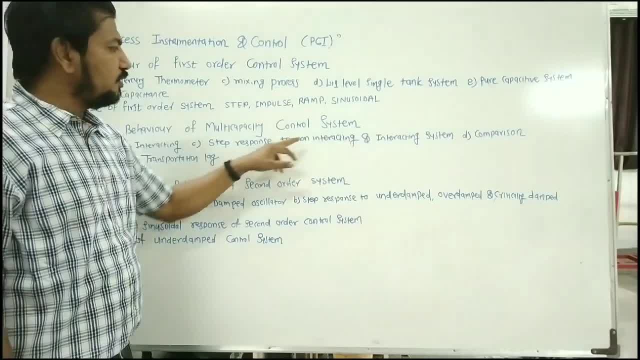 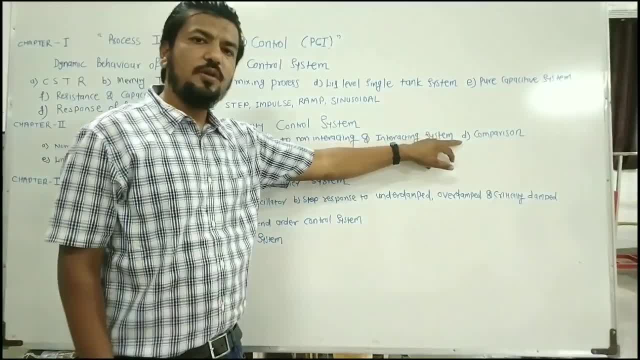 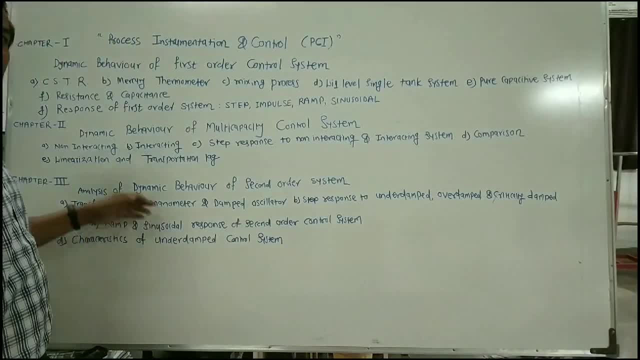 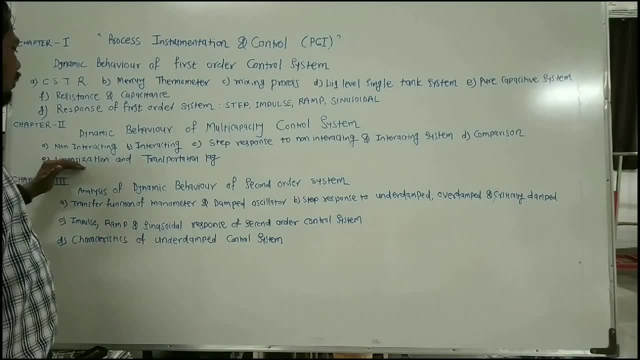 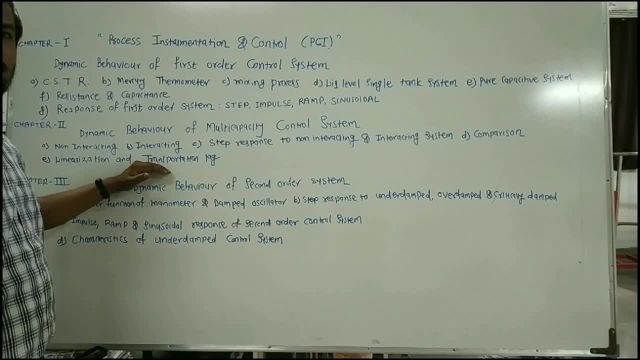 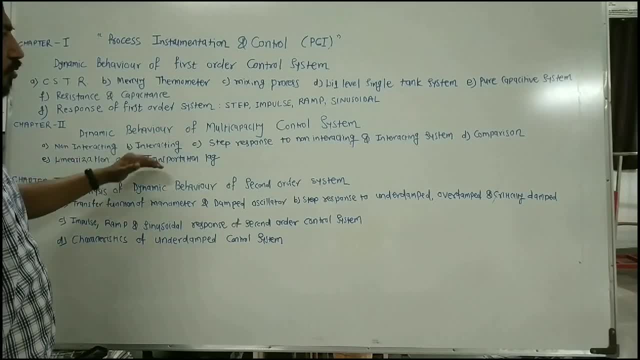 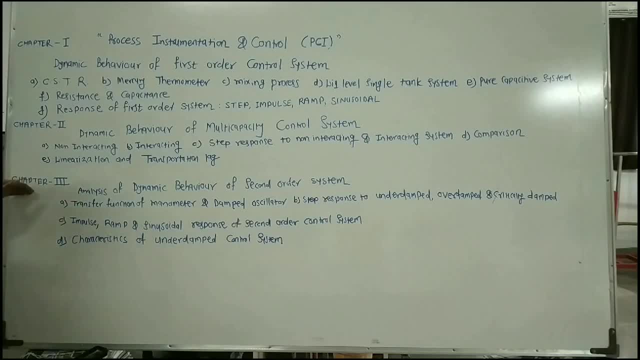 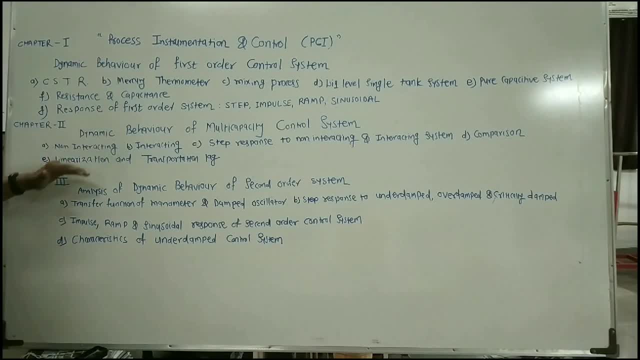 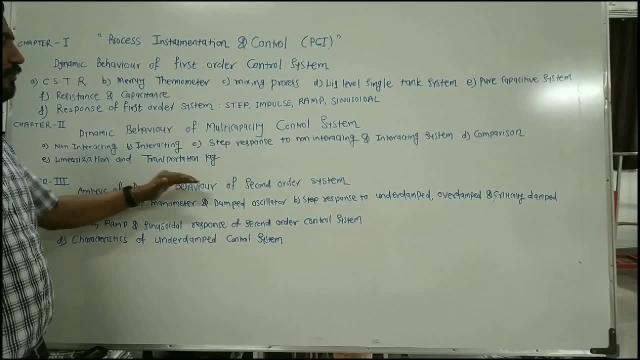 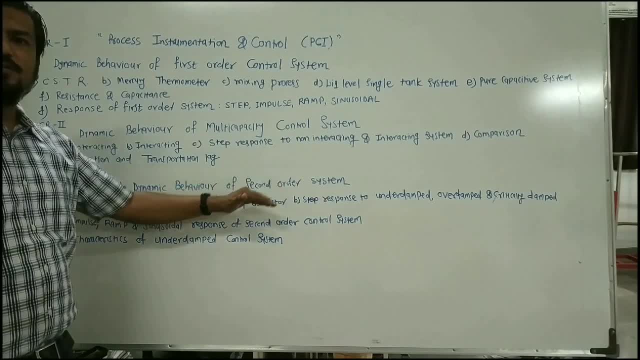 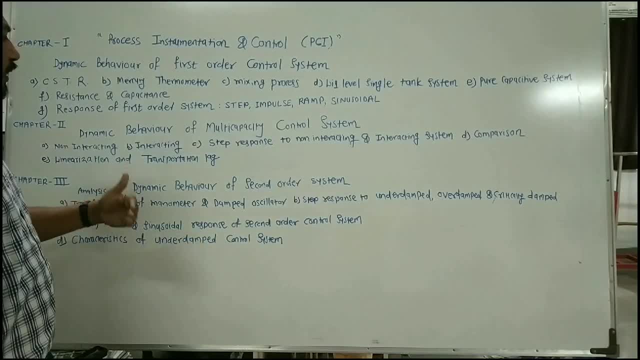 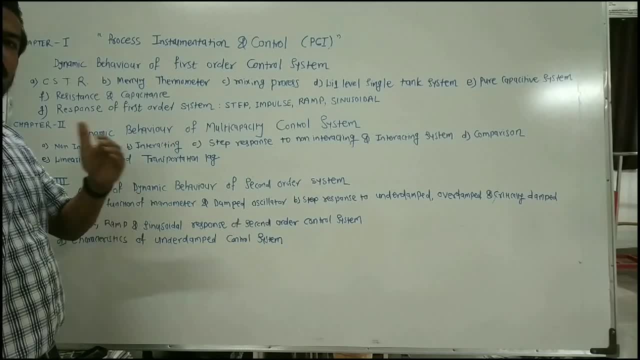 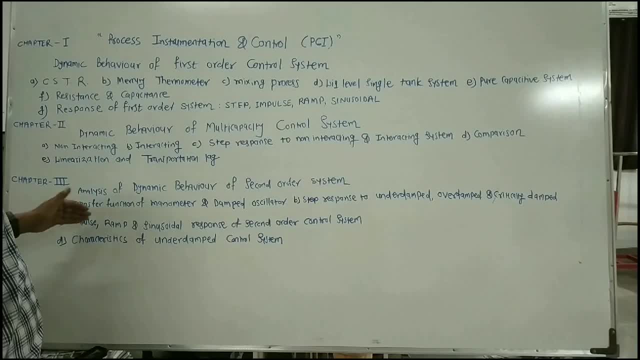 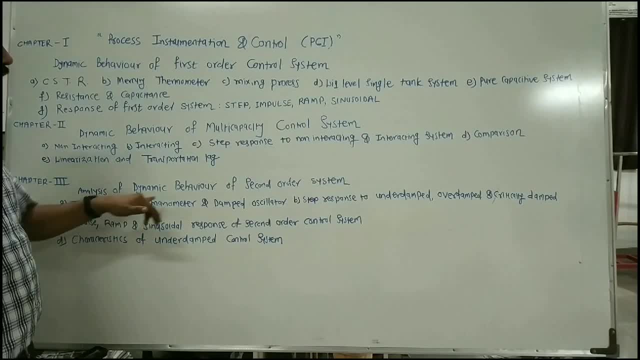 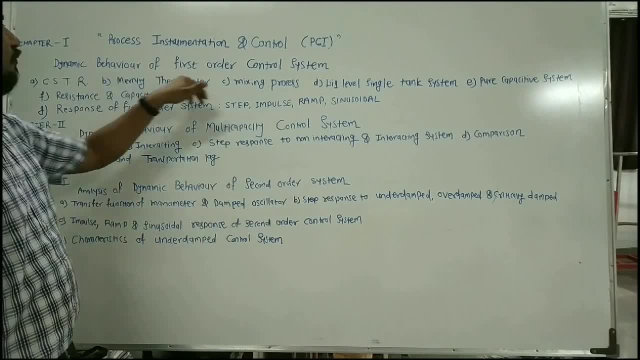 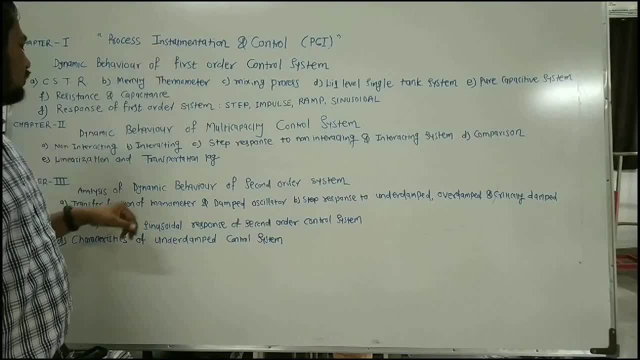 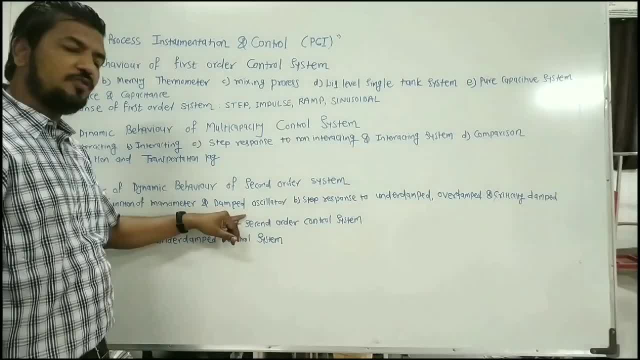 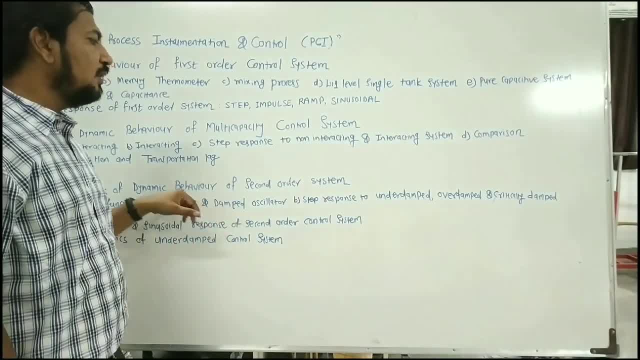 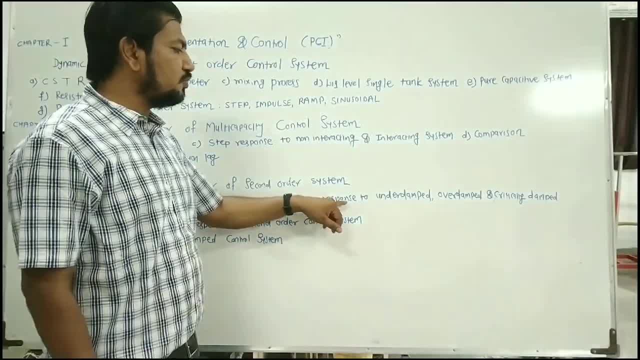 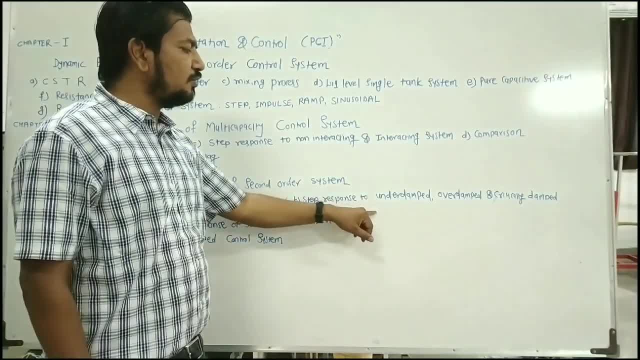 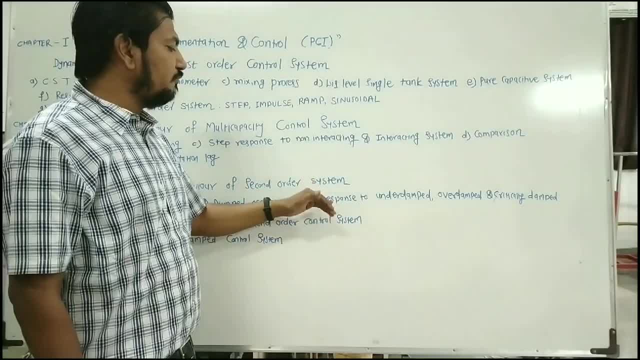 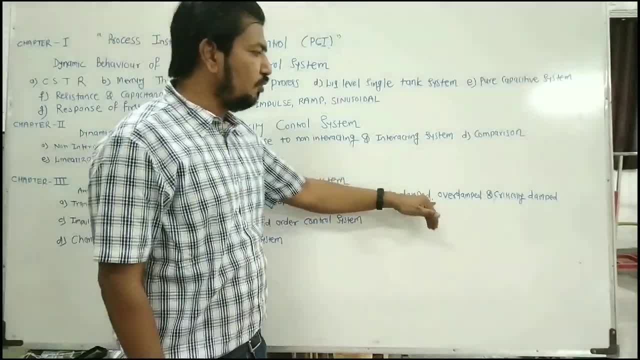 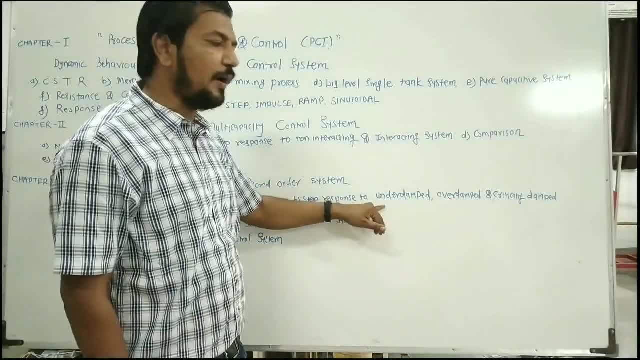 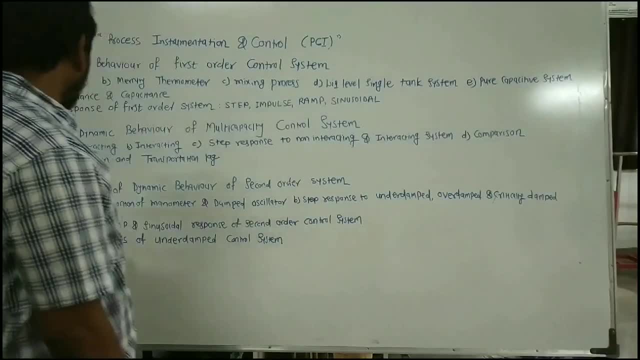 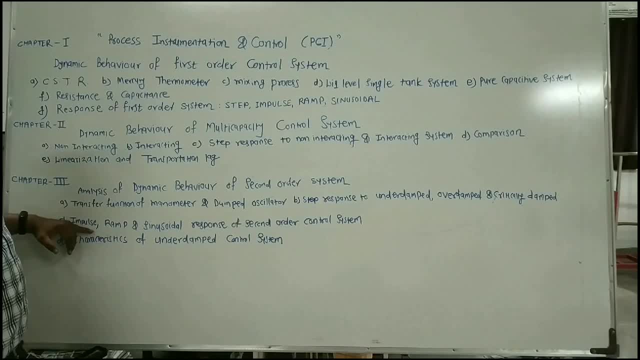 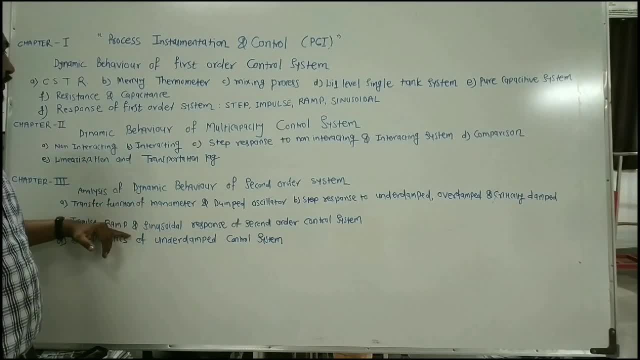 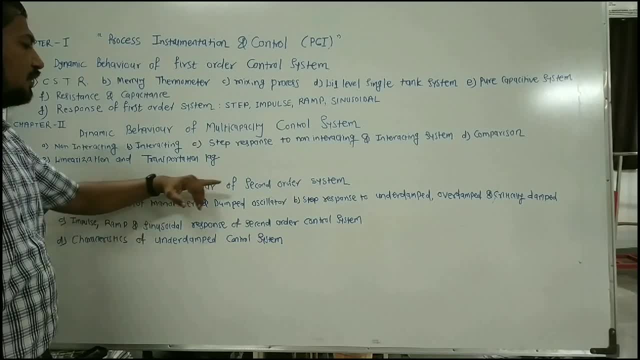 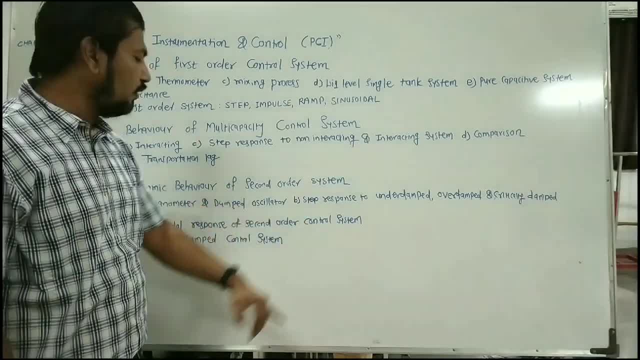 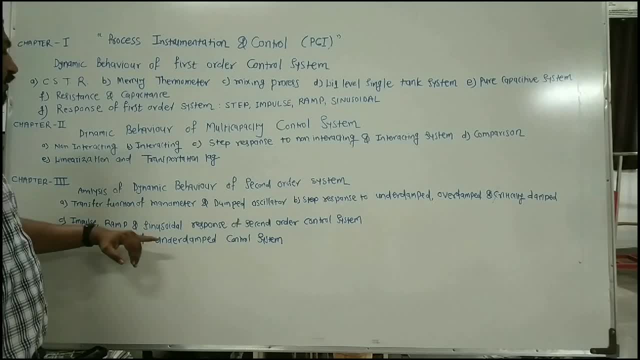 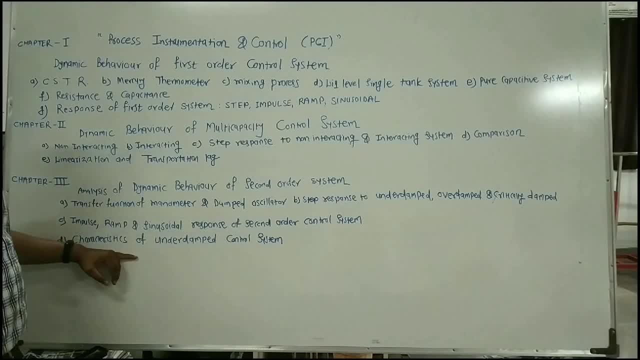 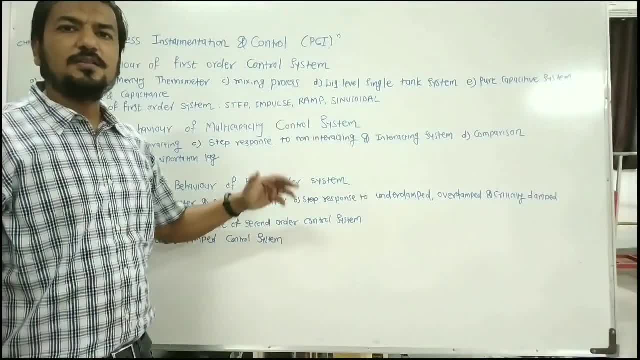 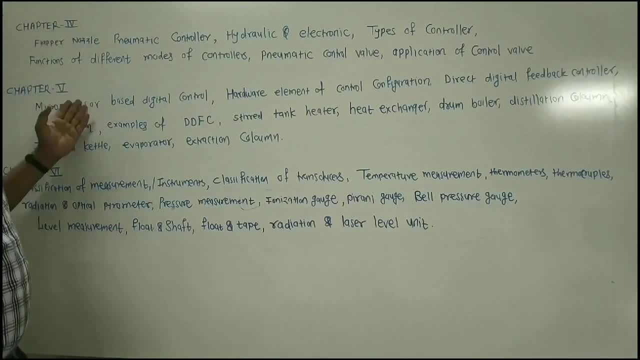 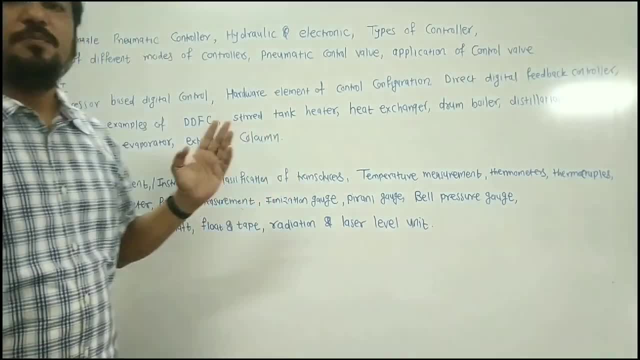 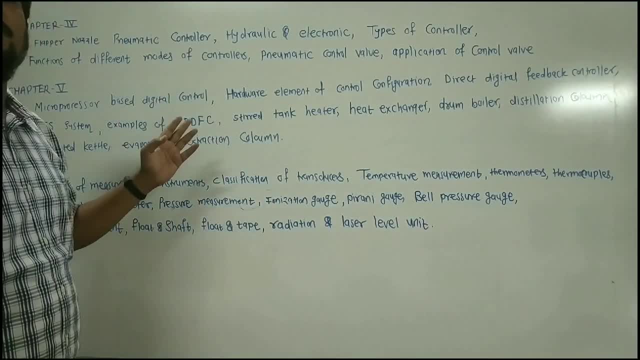 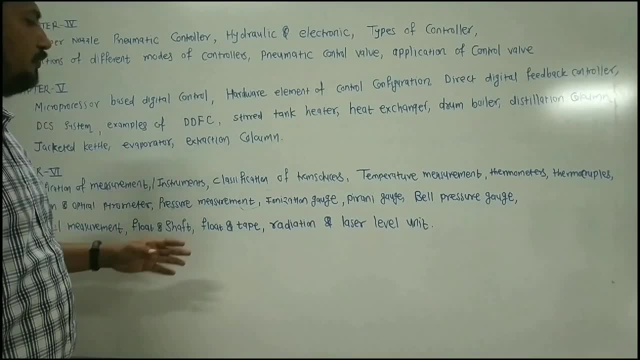 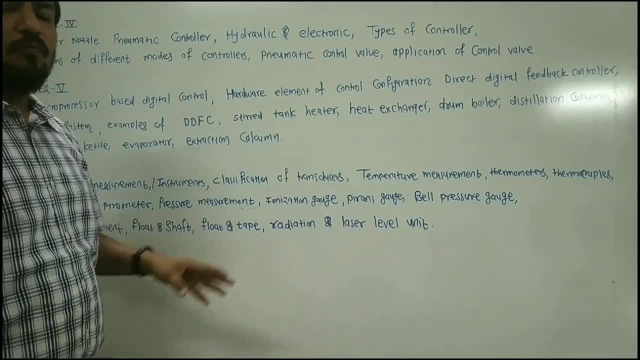 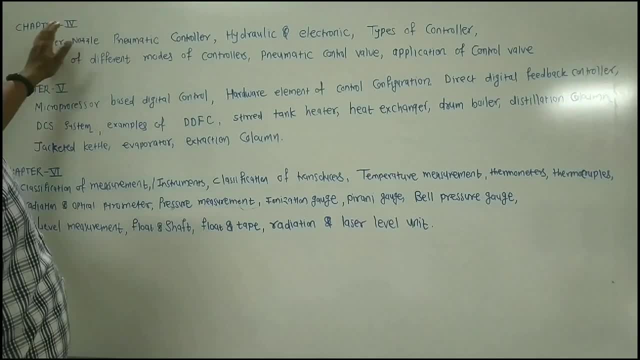 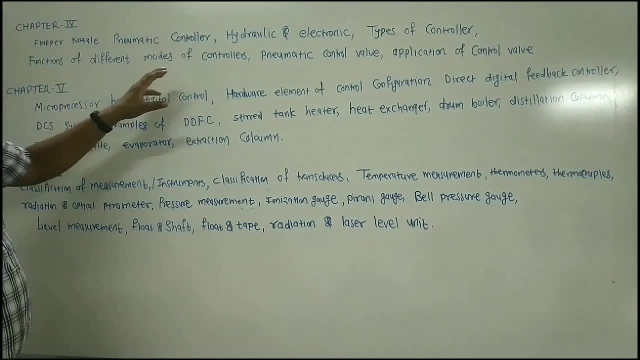 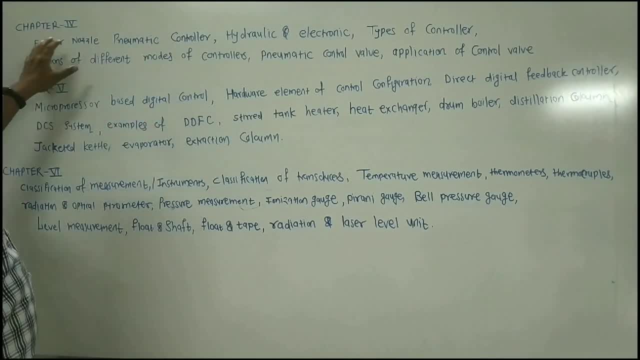 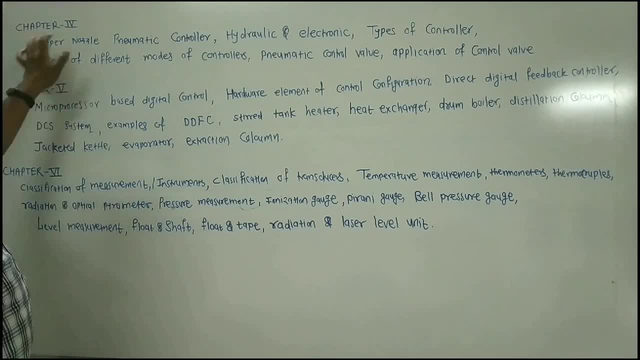 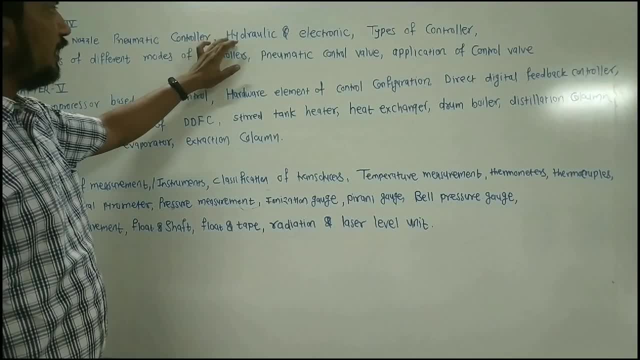 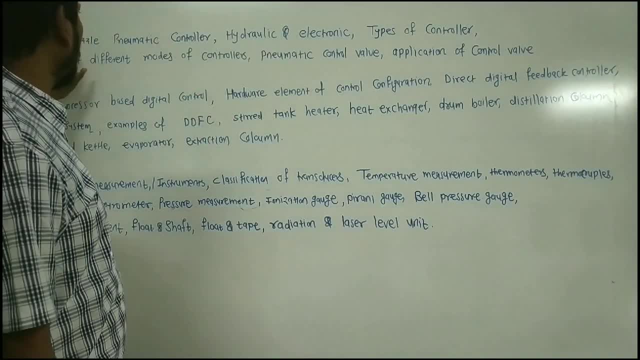 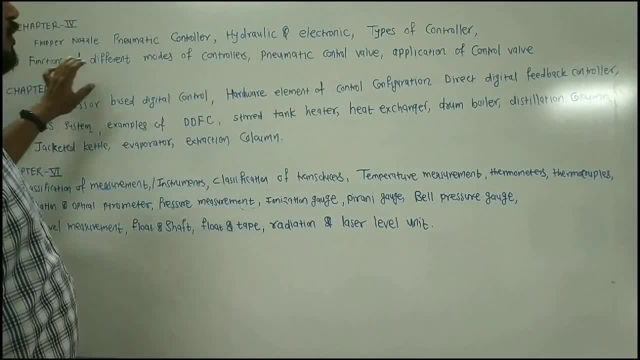 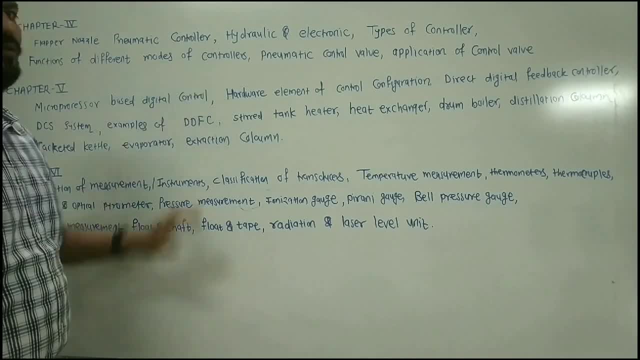 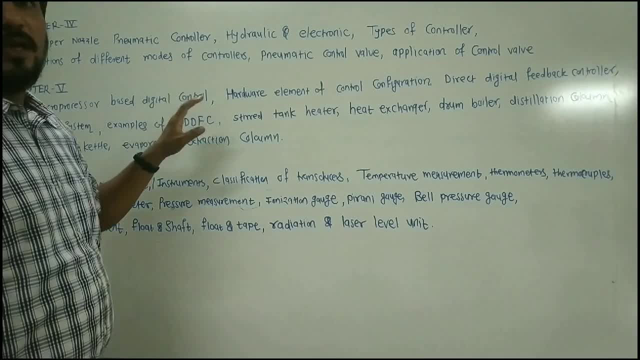 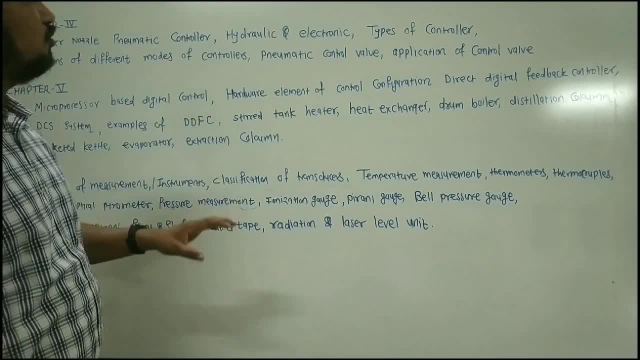 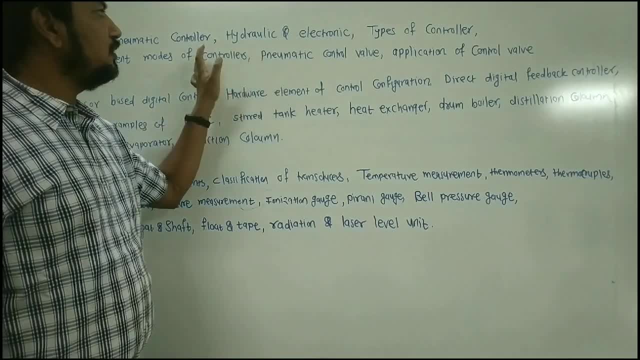 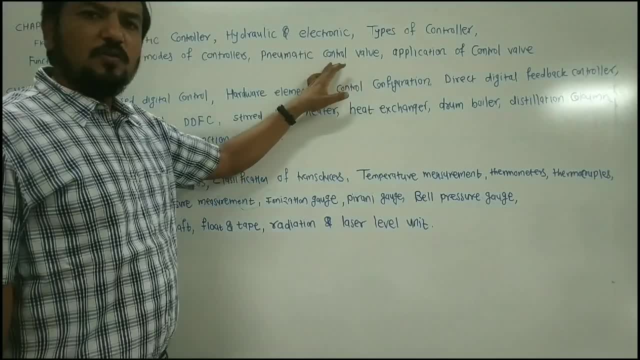 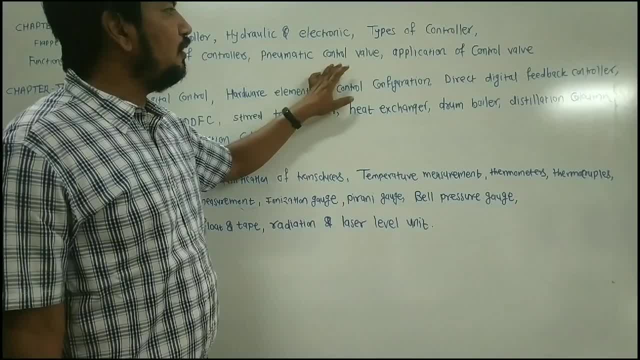 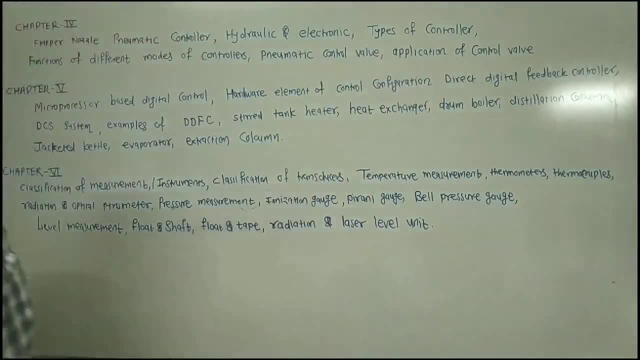 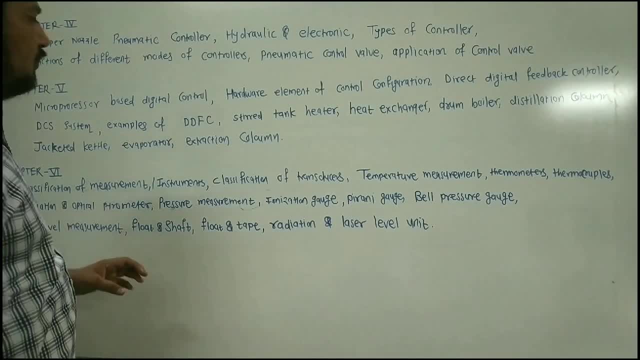 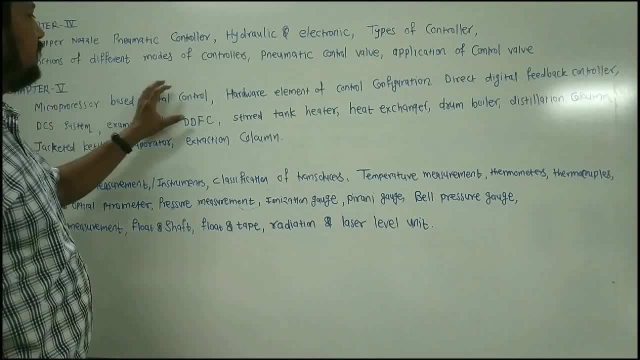 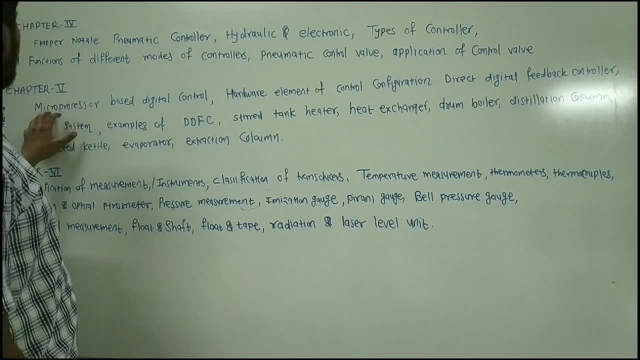 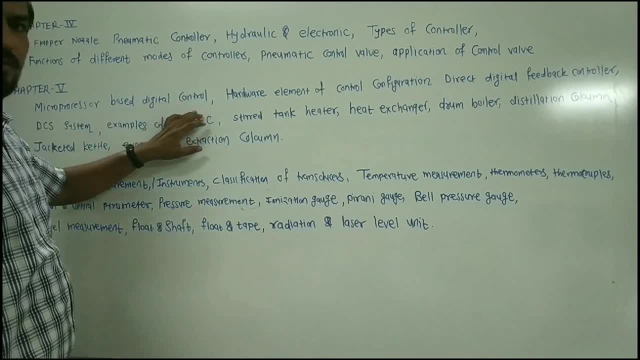 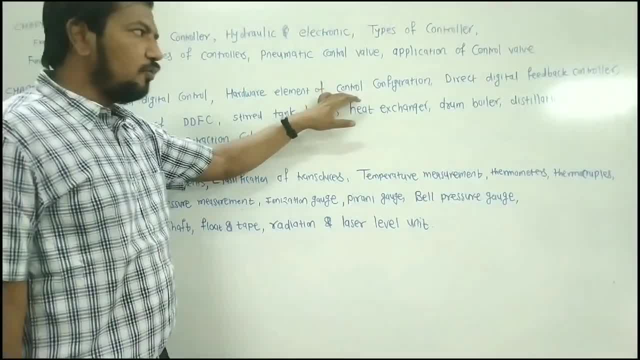 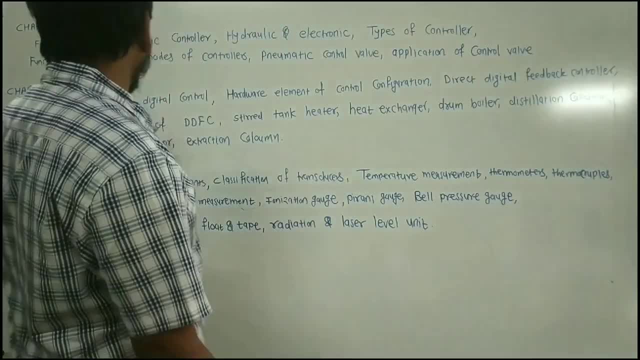 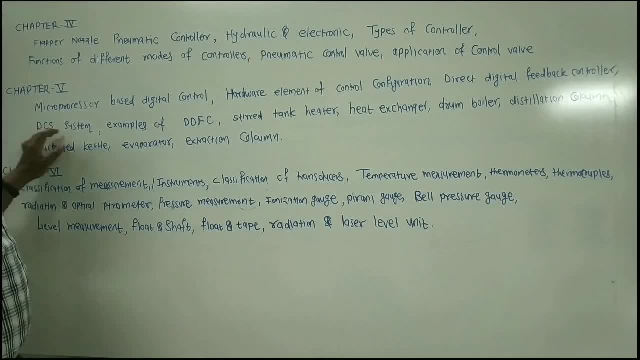 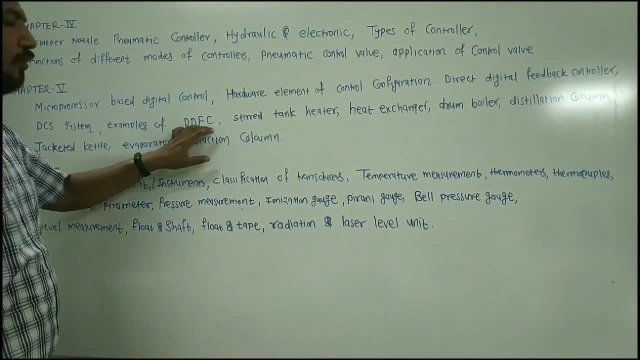 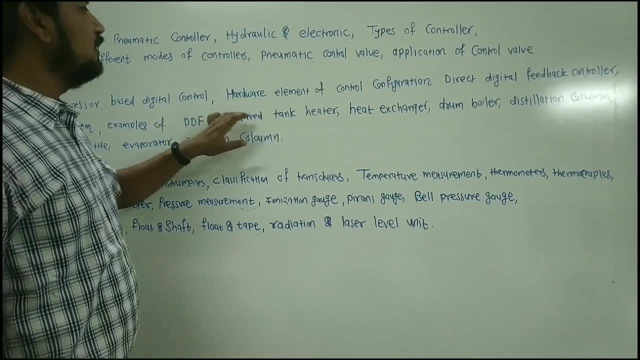 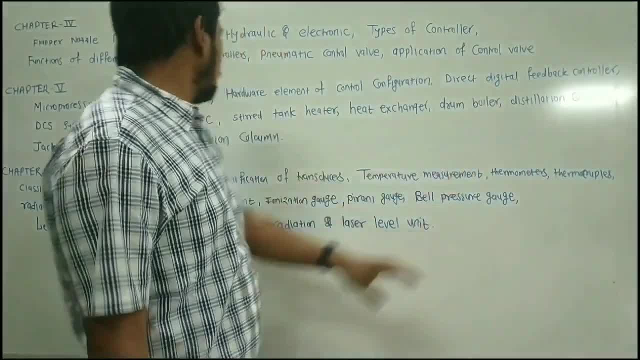 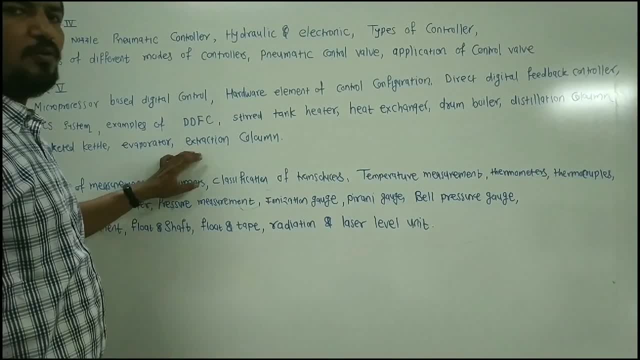 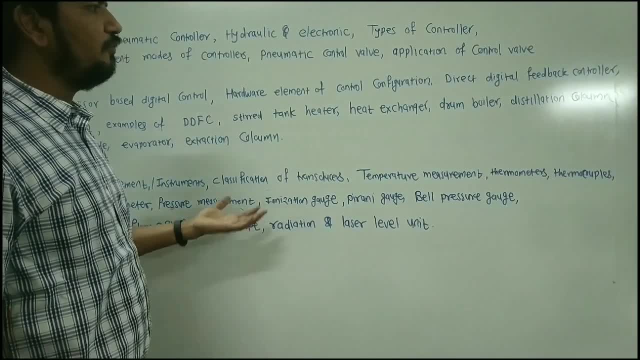 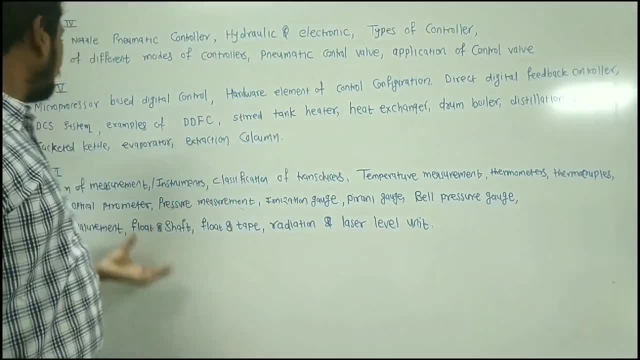 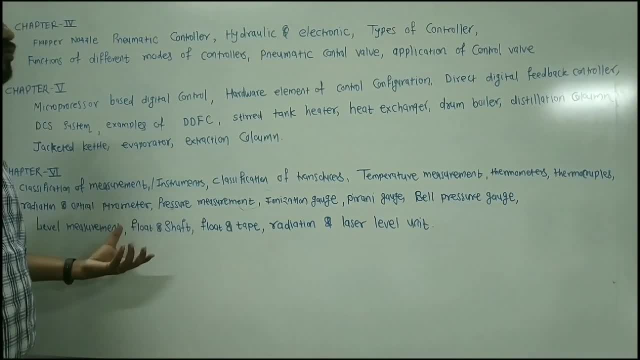 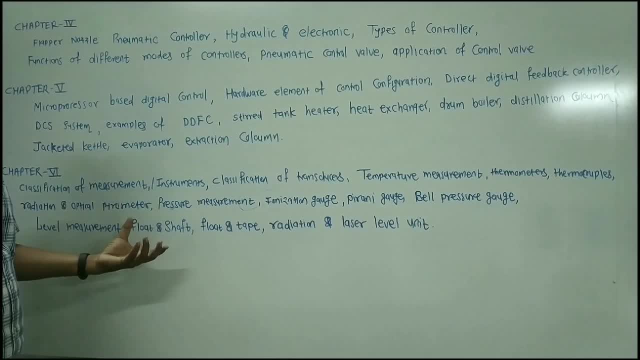 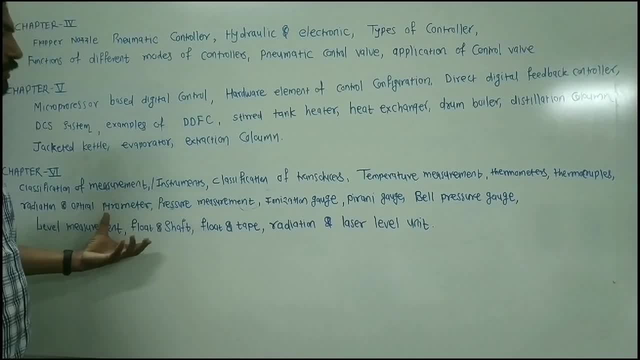 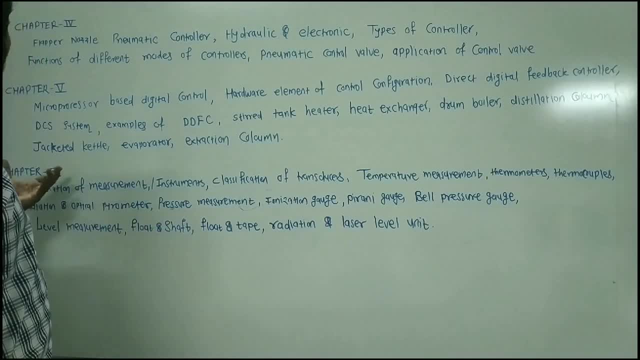 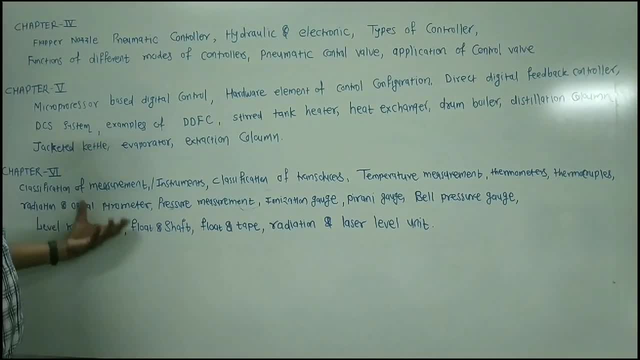 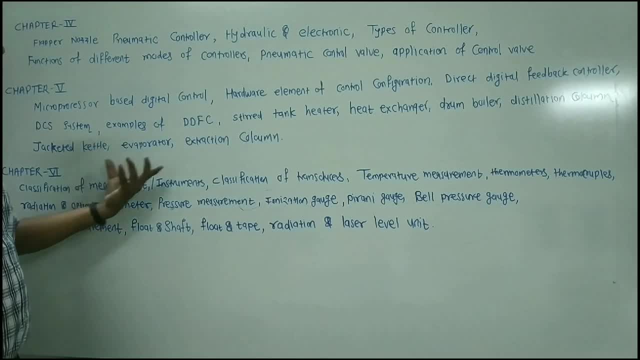 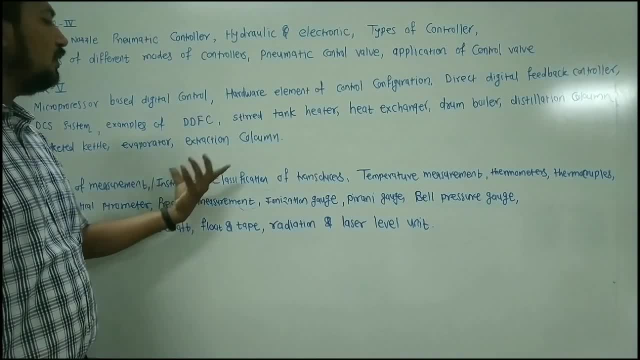 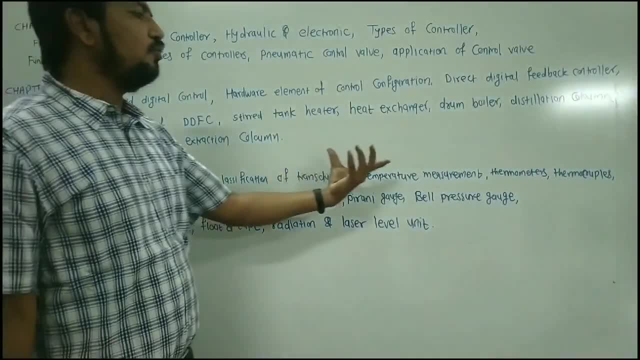 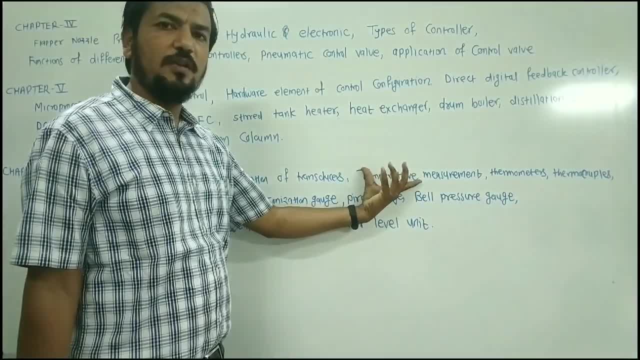 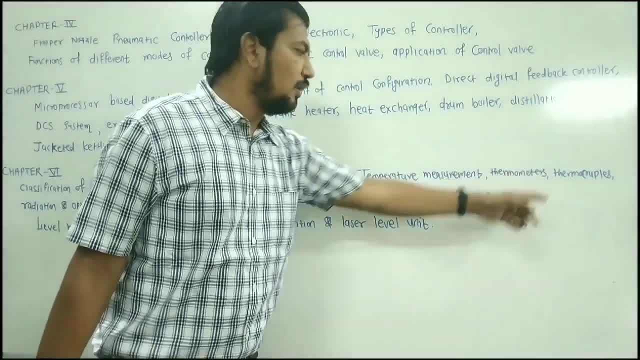 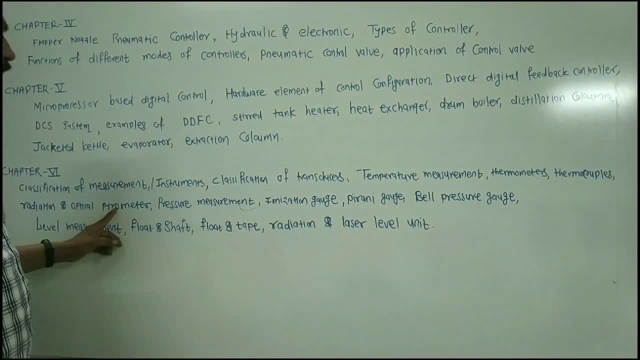 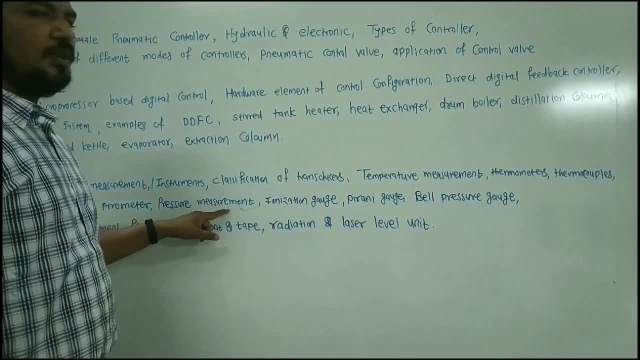 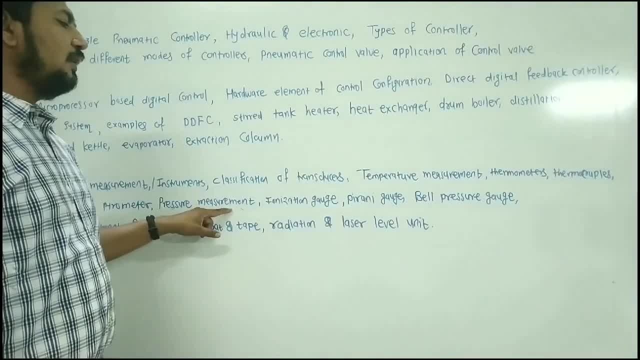 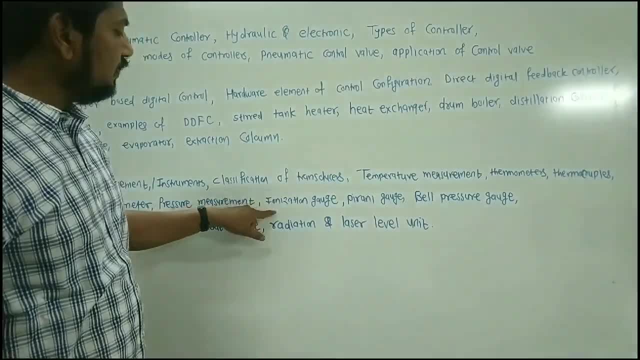 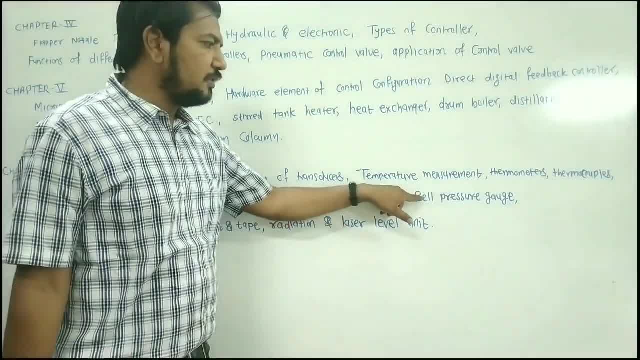 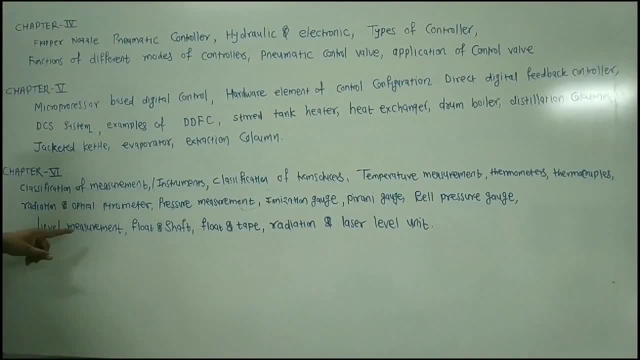 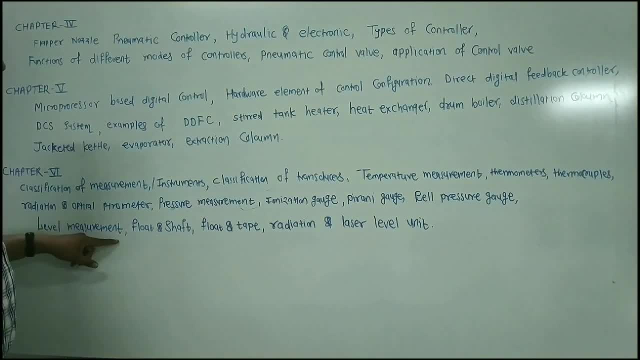 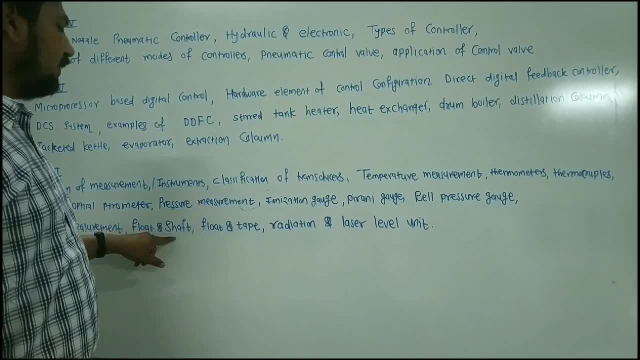 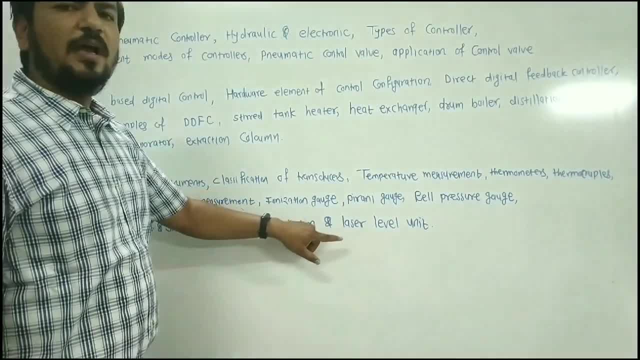 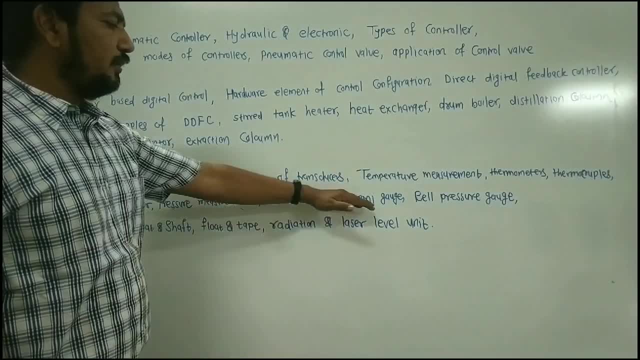 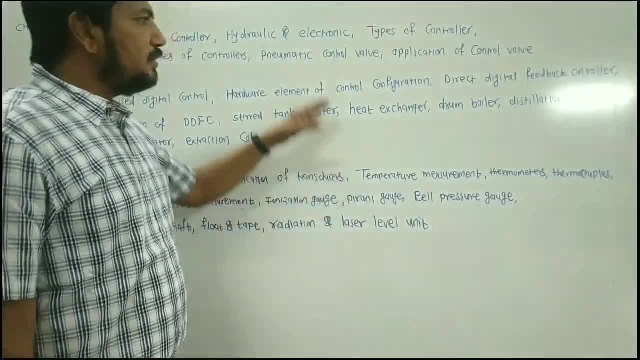 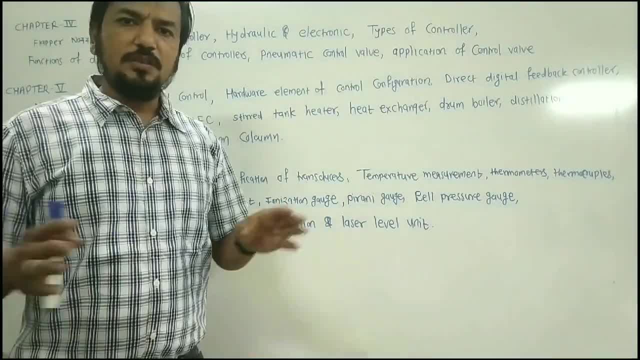 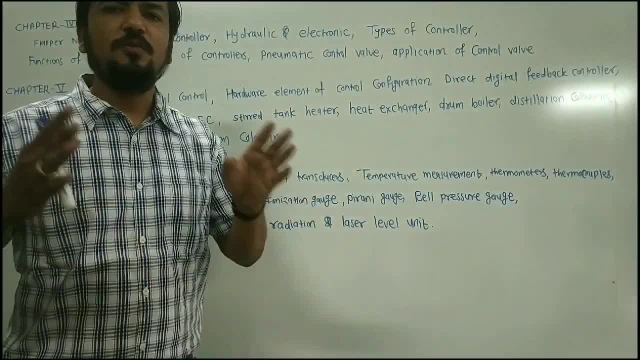 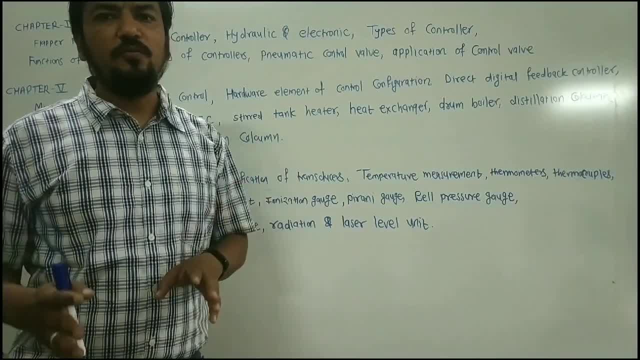 Then you have to determine the transfer function of the non-interacting control system. Then you have to determine the transfer function of the non-interacting control system. Then you have to determine the transfer function of the non-interacting control system. the Pune University, Only the different. 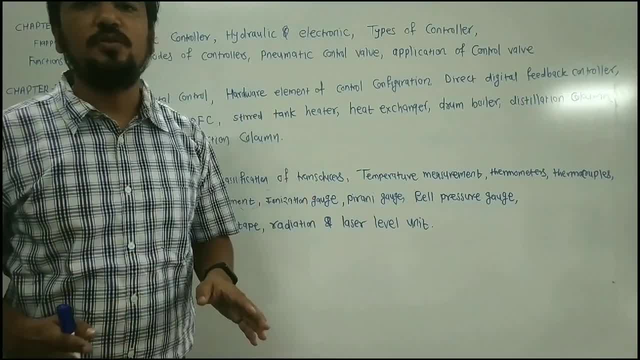 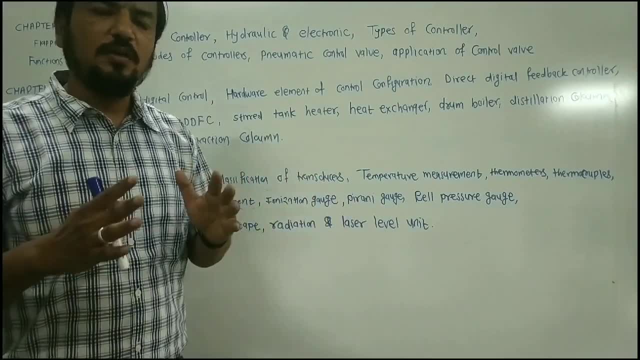 these three universities is the weightage given to the part of the instrumentation. In RTMU University, more weightage is given to the control and all the part of the instrumentation is included in only a single unit, while in other universities the section B or the chapter number.